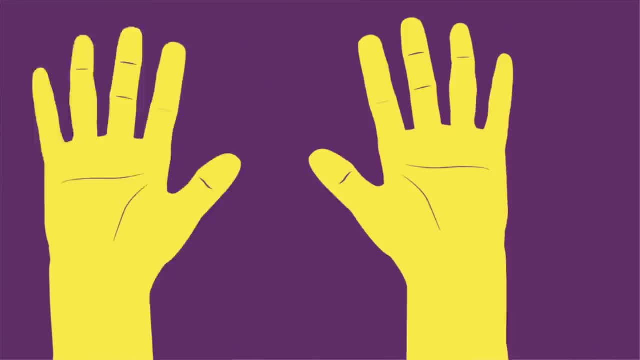 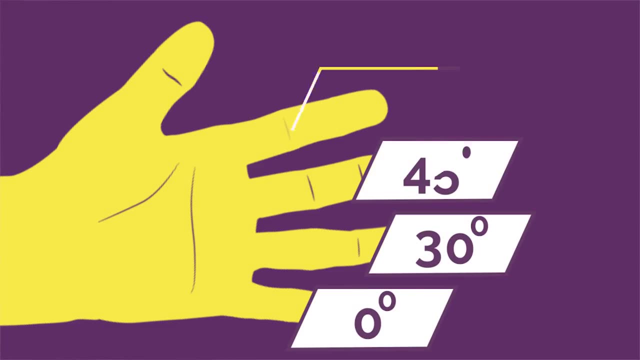 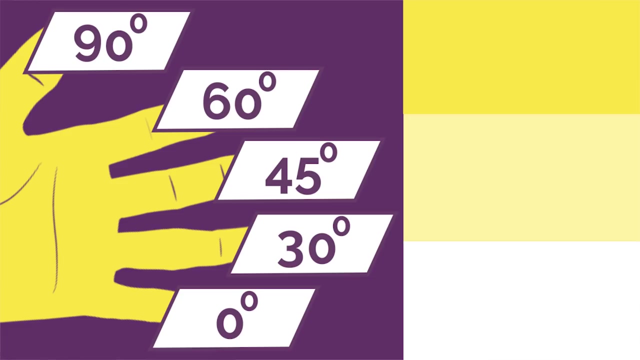 that table of values. Take either hand, with your palm facing towards you, and label your little finger as 0 degrees, your ring finger as 30, middle one as 45,, 60 and your thumb as 90 degrees. To make this work, you just need to remember to square root the number. 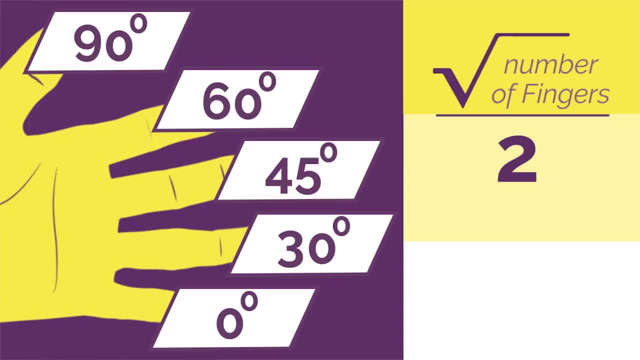 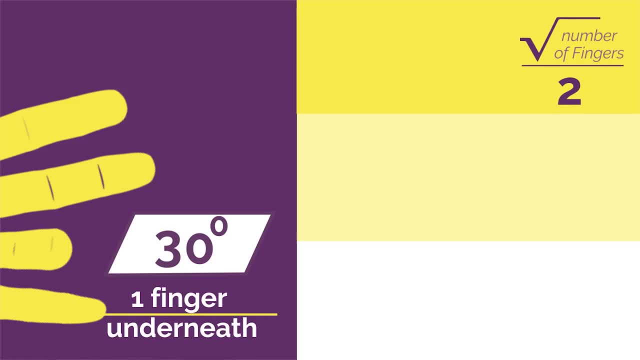 of fingers and divide by 2.. So if we wanted sign 30, we'd bend down our 30 degree finger and you just have your baby finger underneath. So sign 30 is square root 1 divided by 2, because there's only one finger underneath which 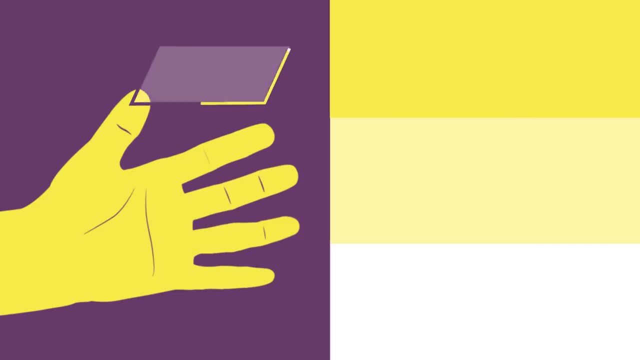 simplifies to a half. If we wanted sign 90 degrees, you'd bend down your 90 degree thumb and so you have 4 fingers underneath. So sign 90 is square root of 4 divided by 2, which simplifies to 1.. 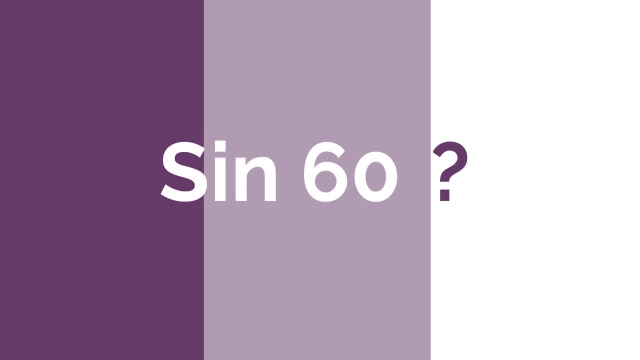 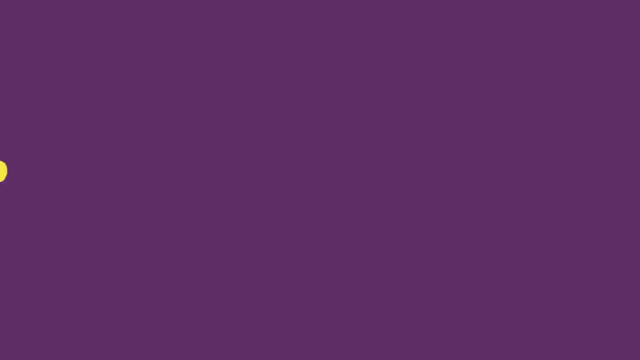 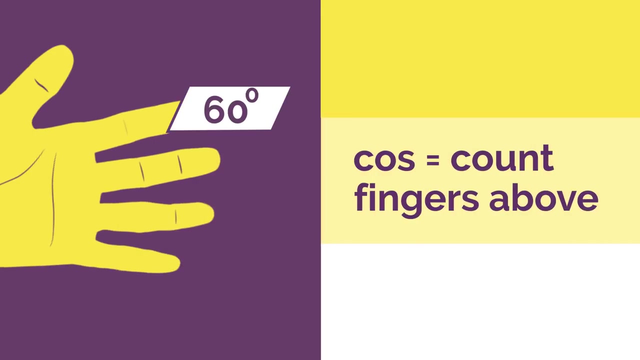 What would sign 60 be? Work out the answer and click here when you're ready to check. Did you get square root 3 divided by 2?? For cos, we just count the fingers above instead of the ones below. So for cos 60, bend down your 60 finger and count the fingers above. 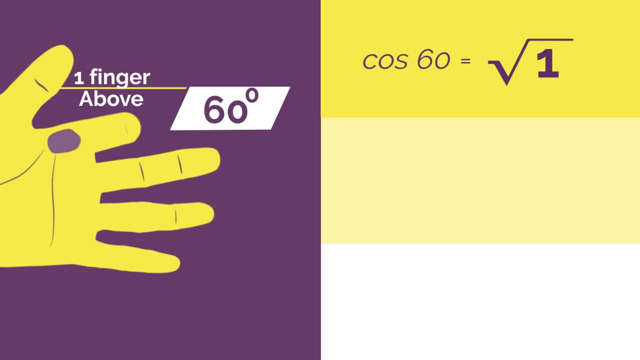 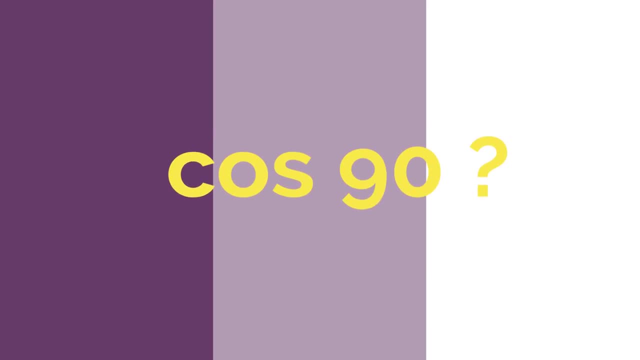 1.. So cos 60 is square root 1 divided by 2.. What would sign 60 be? Work out the answer and click here when you're ready to check. Did you get square root 2 divided by 2?? For cos 60, bend down your 90 degree thumb and 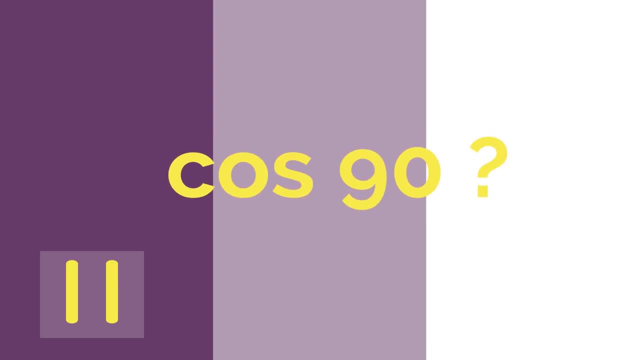 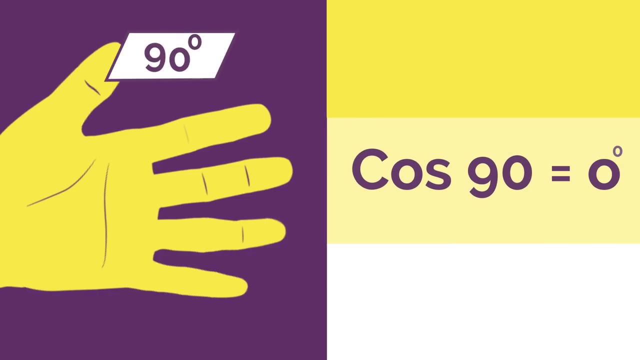 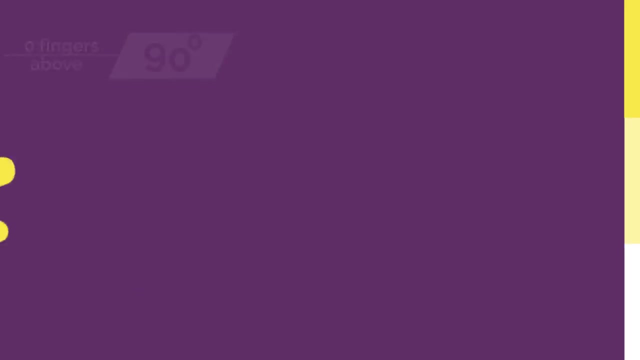 3 fingers above. So sign 90 is square root of 4 divided by 2, which simplifies to one. What would sign 60 be? Work out the answer and click here when you're ready to check. Did you get square root 4 divided by 2?? For cos we just count the fingers above instead. 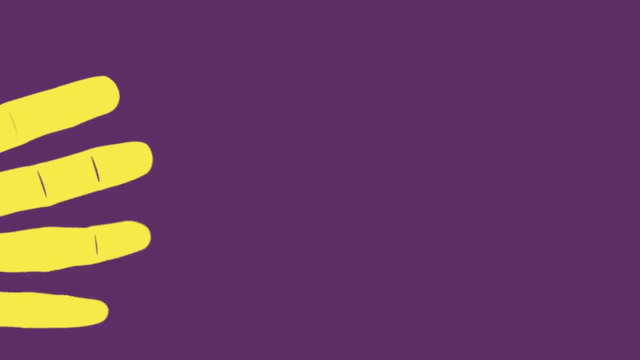 of the ones below, What would sign 60 be? Work out the answer and click here when you're ready to check. Did you get square root 0 divided by 2?? For cos we just count the fingers above instead, we still count fingers, but there is just one extra little twist. the same as for. 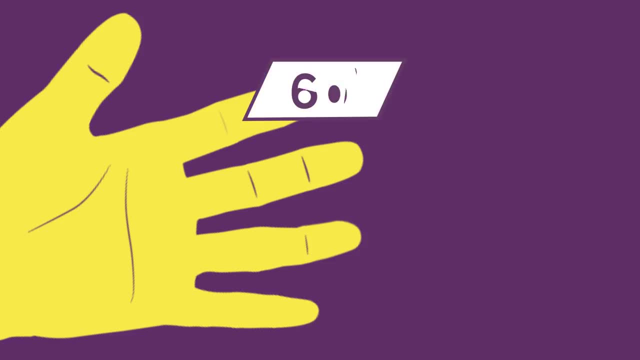 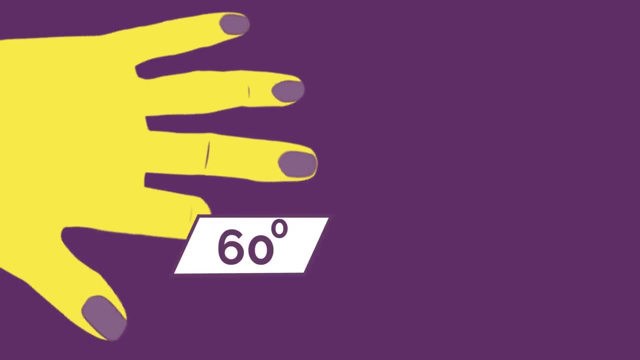 sine and cos bend down the angle finger. so let's find tan 60. let's bend down our 60 degree finger. we've got one cosine finger above and three sine fingers below. for tan, we flip our hand over and we have three sine fingers above and the.